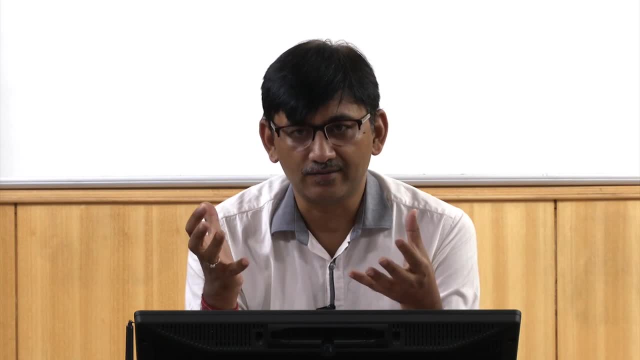 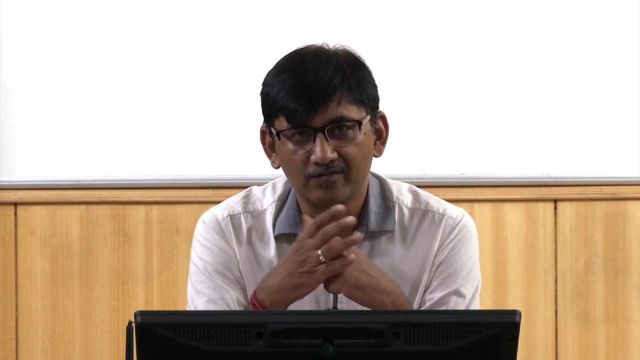 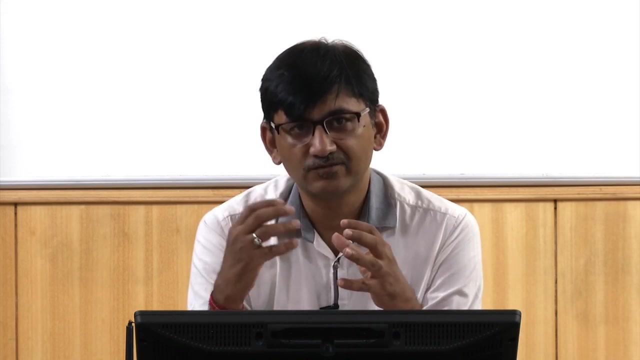 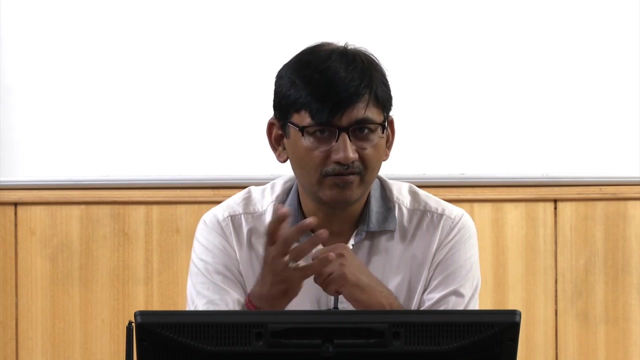 So you can understand that when, for example, you must have seen the formation of ice from water when you keep water in the freezer. So there has to be some Some place where the nucleation is started and that nuclei is growing. So always, whenever you have any kind of transformation, there has to be some nuclei which is taking. 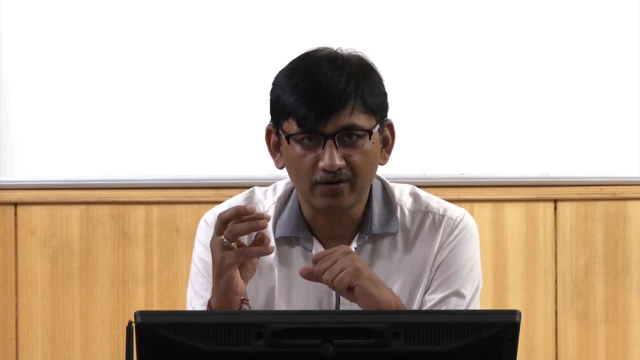 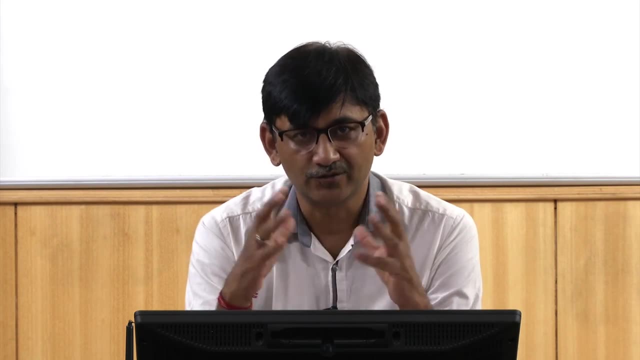 place or some nucleation event has to take place, and that nuclei will then grow and then it will take up the whole space. So from liquid to solid, or you can have solid to solid transformation, as we saw in case of steel, from austenite to ferrite or austenite to pearlite, or from solid, and that means from. 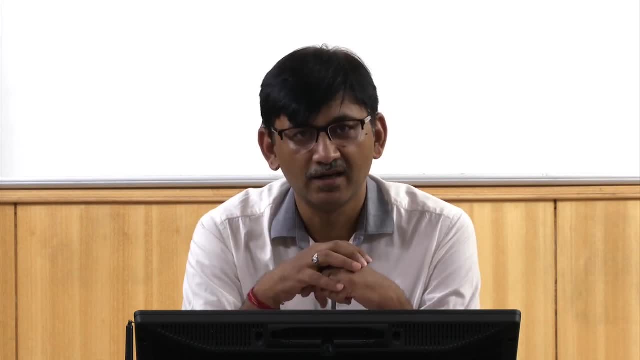 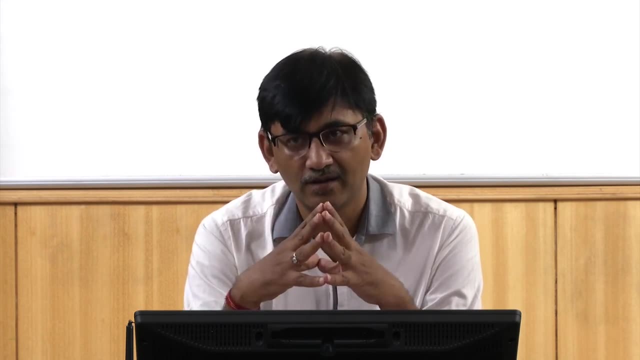 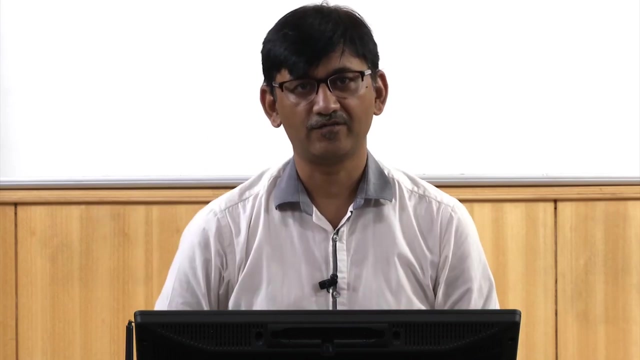 liquid phase to solid phase during solidification. So in this all processes there has to be some formation of a nuclei and then nuclei will grow In solidification. for example, the vessel in which you are pouring the liquid metal, that vessel wall itself act as a site. 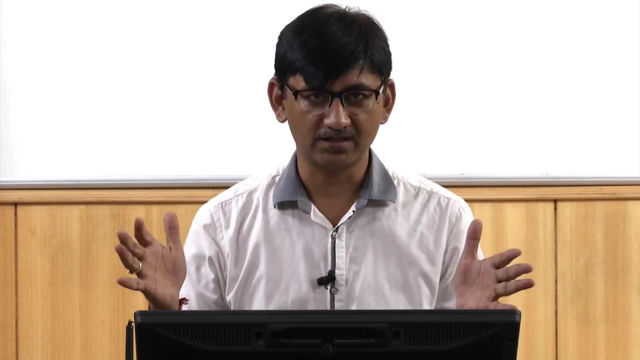 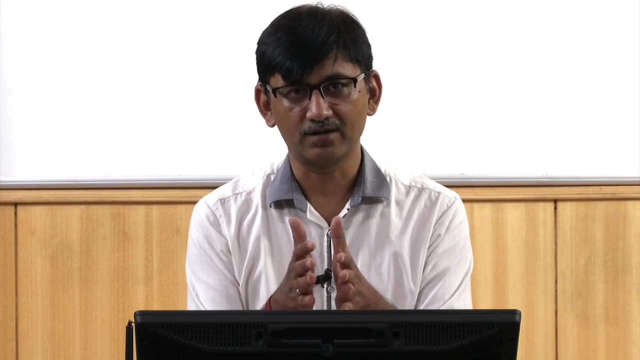 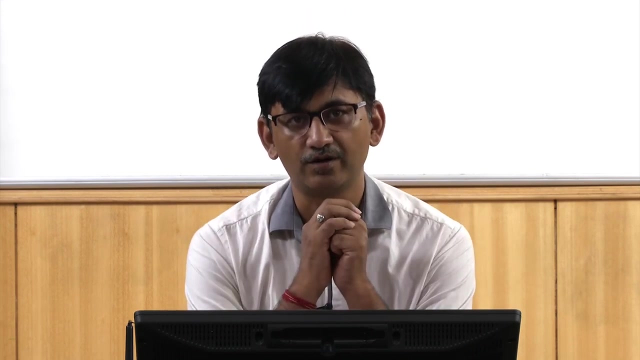 Where the nucleation will take place. So nucleation starts from the wall and then the growth goes inside the molten metal, inside the, basically inside that vessel, and then the whole liquid metal will solidify. and that is what, if you do a close examination of formation of ice. 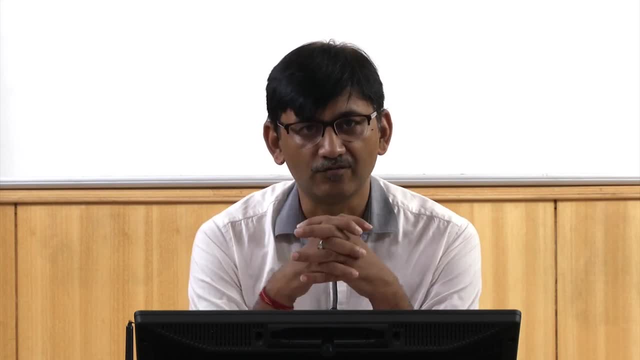 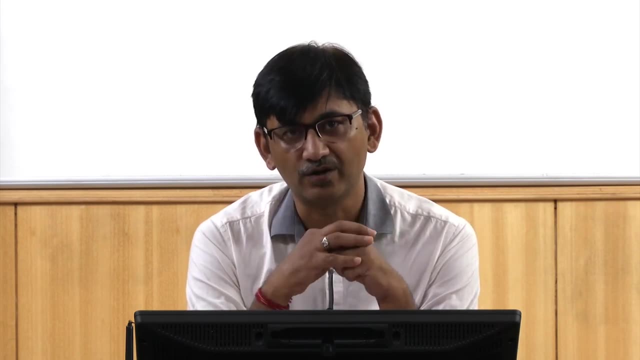 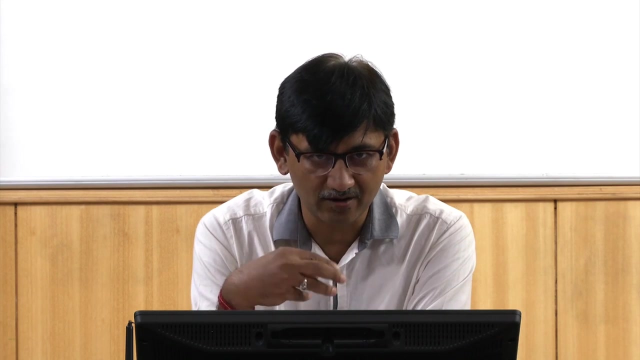 in your freezer, you will see that it is starting from the walls and it is then going inside. the So central part will be the last one to solidify. So that is what is the nucleation and growth process, and from that also we will like to 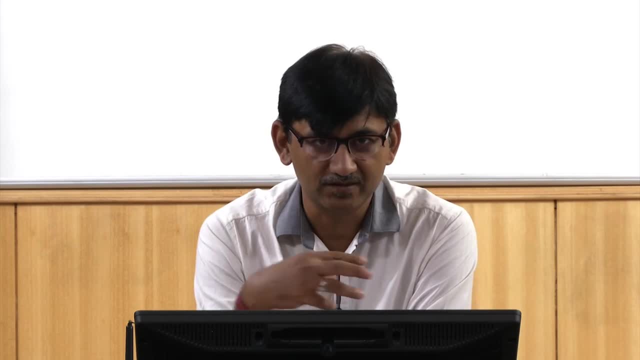 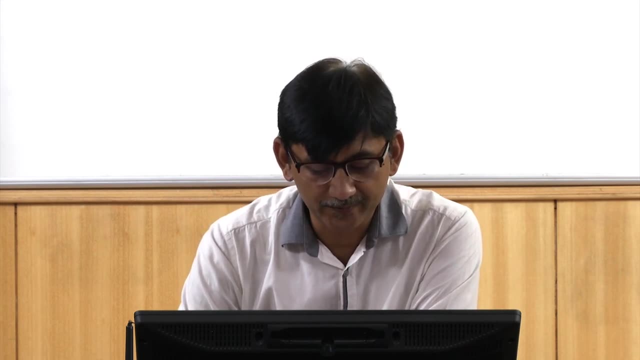 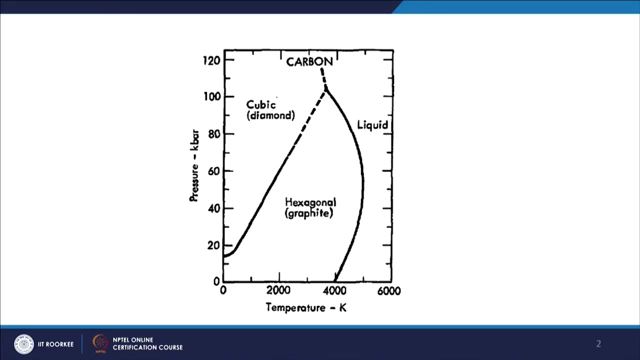 bring the time factor in the whole of this transformation process. So just to again bring the idea of, if you remember when we were discussing initially, that the carbon exist in form of A hexagonal graphite, as you can see here. So you have a hexagonal graphite here and 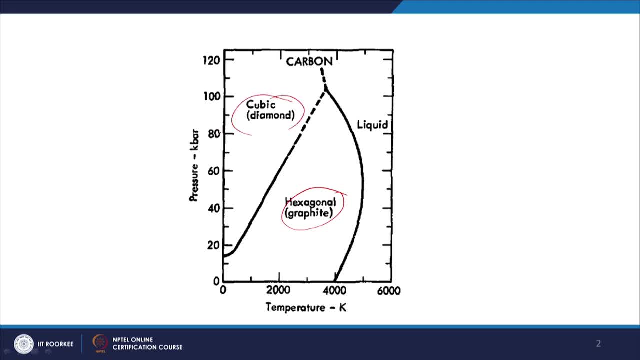 you have cubic diamond here. So if you see, this is a pressure. temperature scale is temperature and pressure. So at lower temperatures and lower pressures means our normal room temperature pressure. actually the diamond is not the stable phase. it actually should transform to graphite maybe. 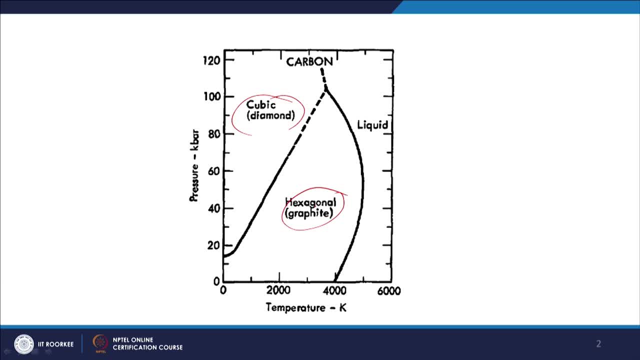 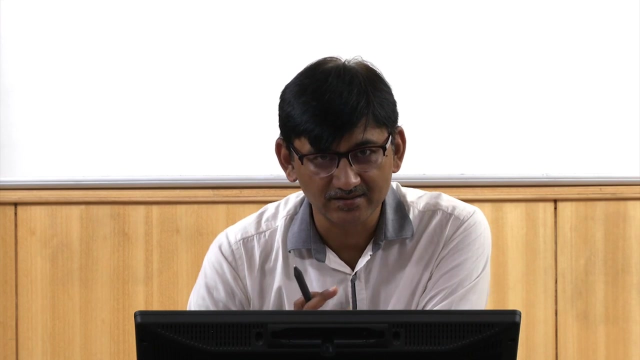 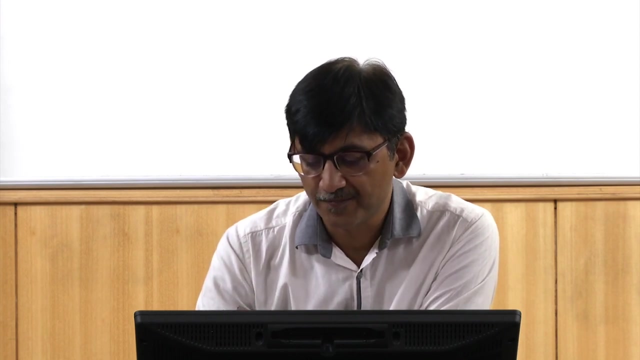 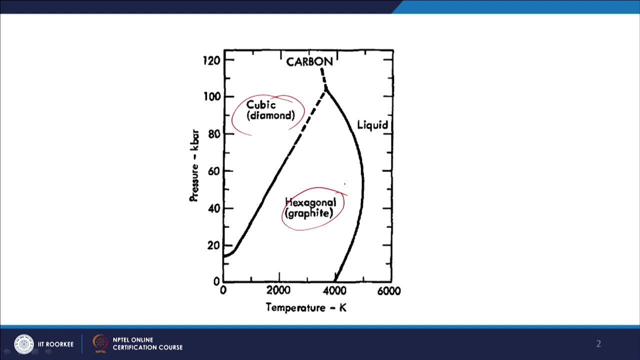 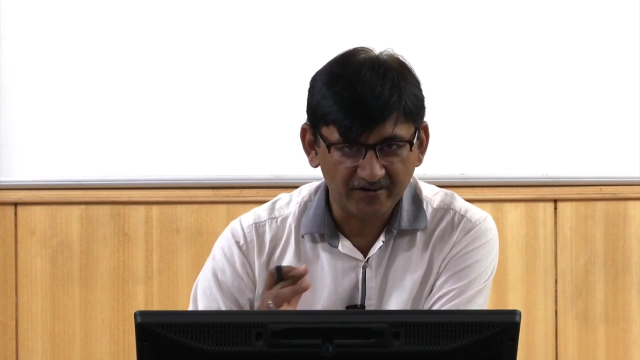 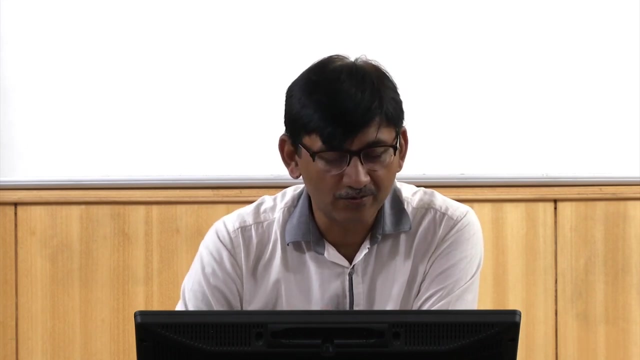 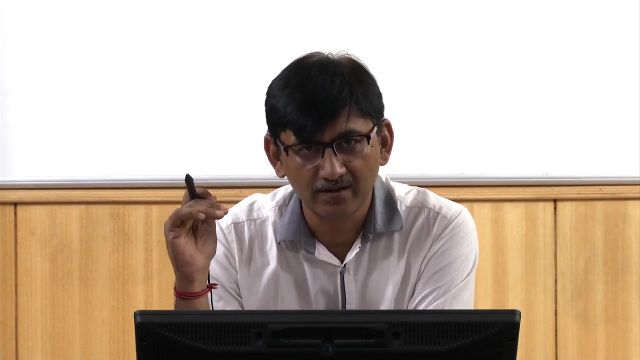 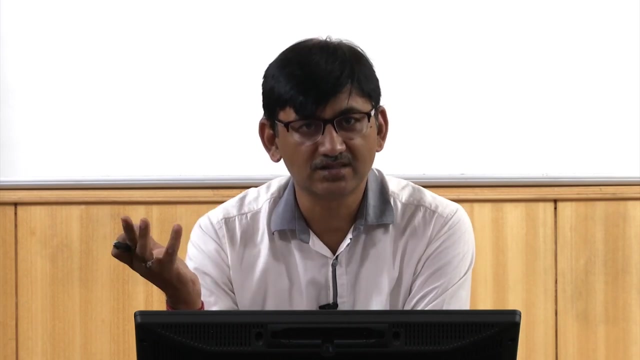 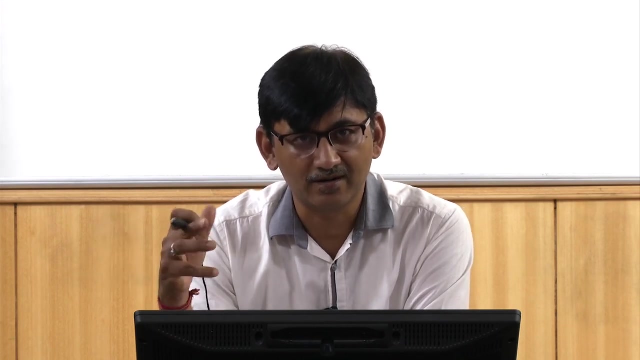 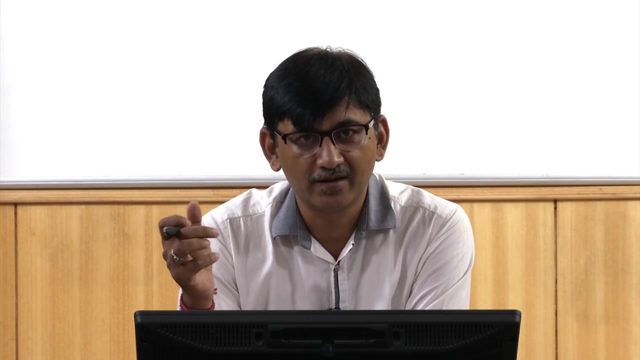 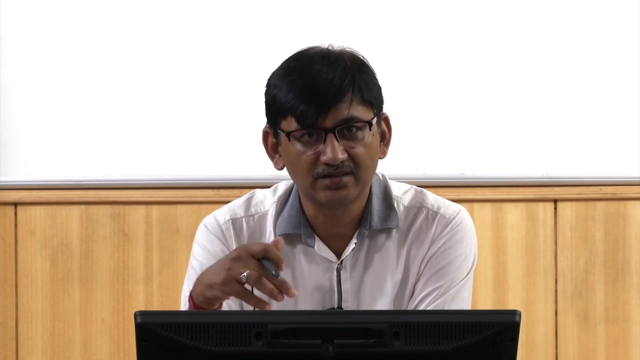 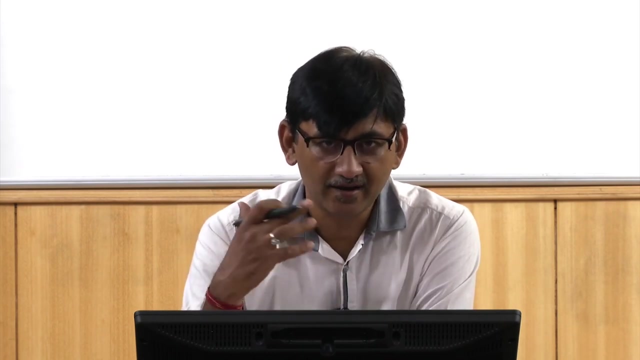 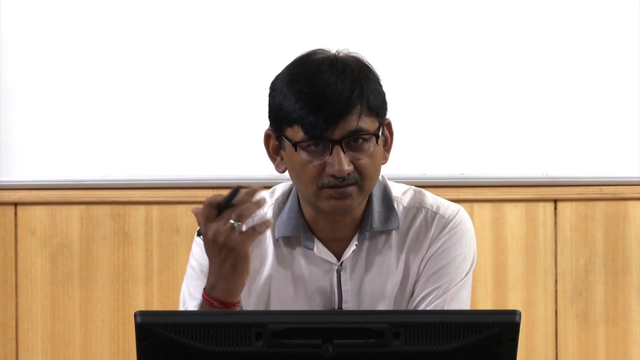 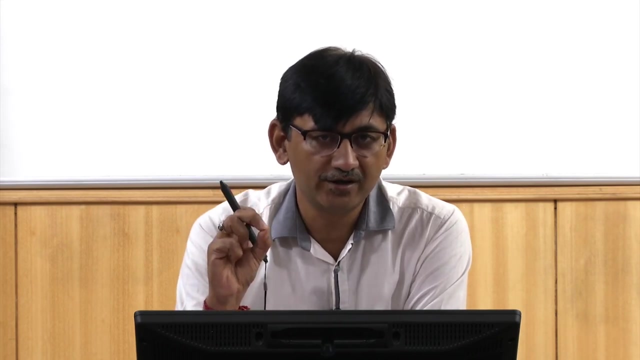 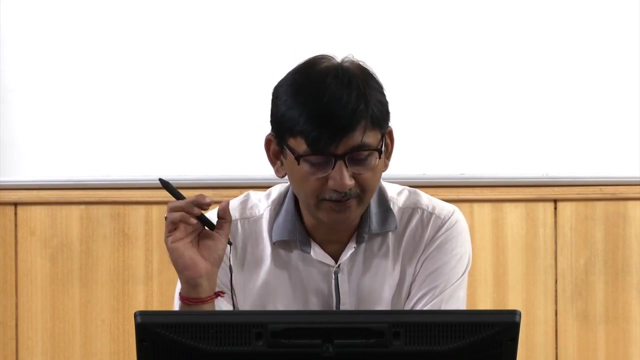 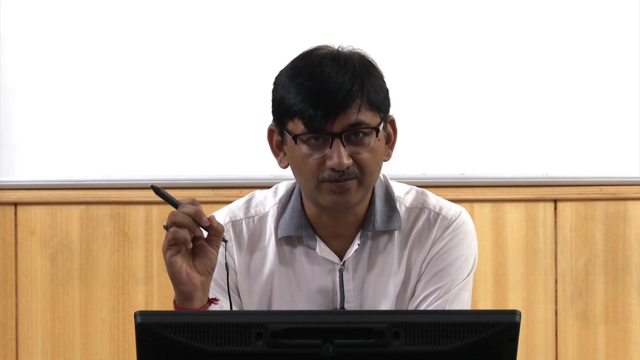 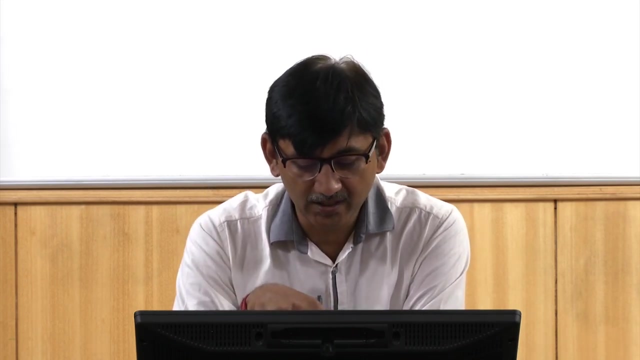 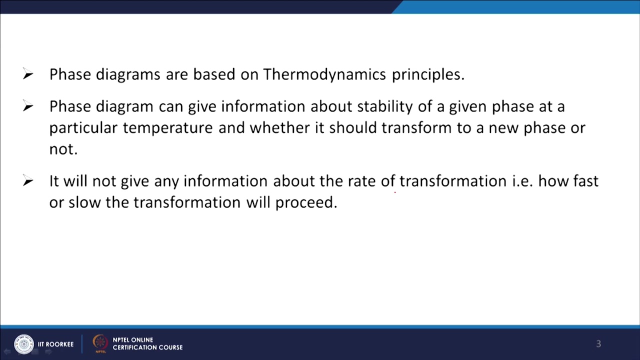 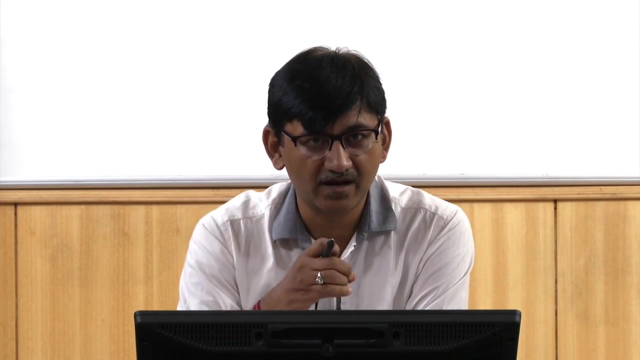 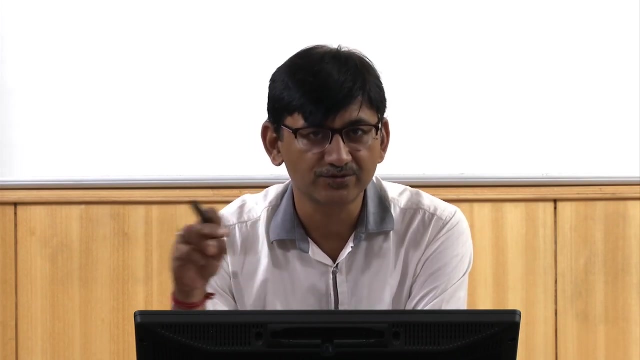 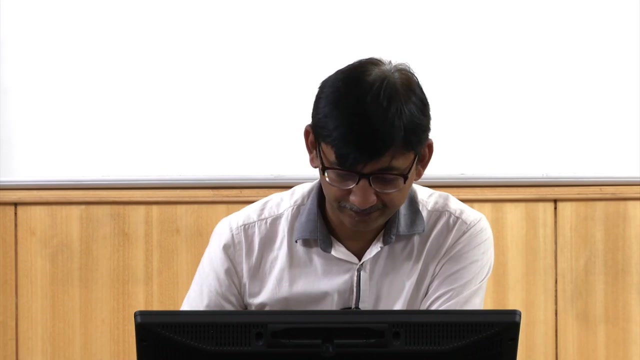 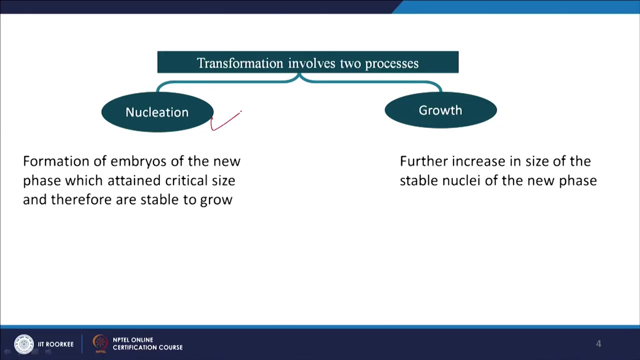 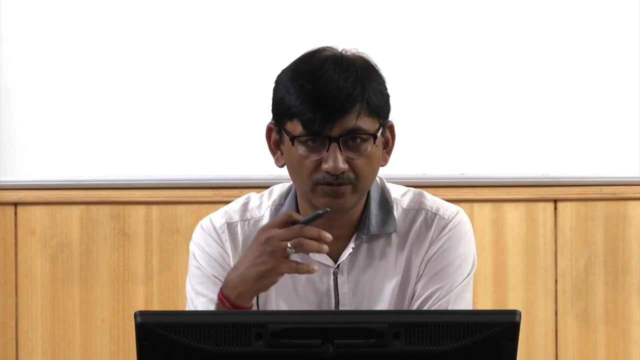 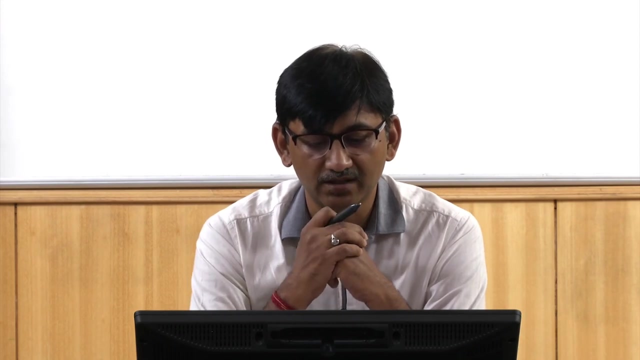 So this phase will change from this particular state to the another state. So if you see transformation, the transformation involves 2 processes. one is nucleation. that means when liquid is transforming into solid or one solid is transforming into another solid, there has to be some nucleation at some point. there has to be some nucleation and then that nuclei. 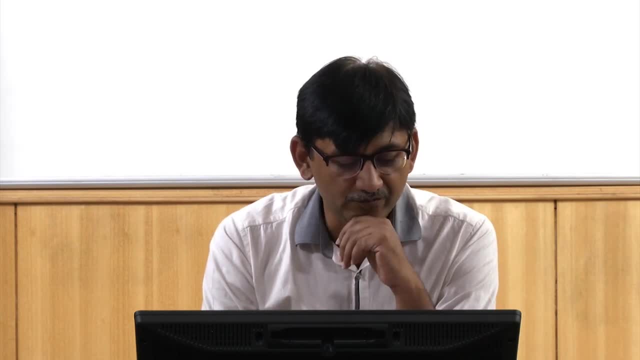 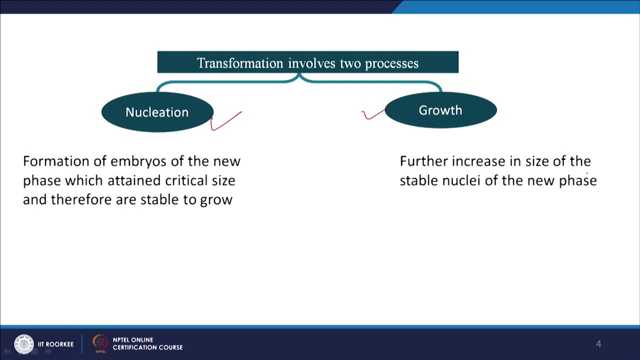 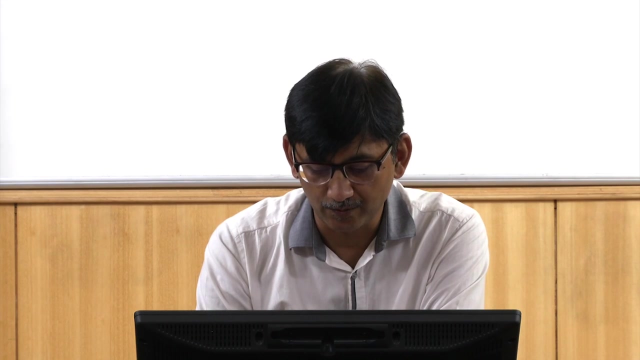 So there has to be formation of mrrio of the new phase which attains critical size and therefore are stable to growth, and then you have a growth process, further increase in the size of stable nuclei of the new phase. So this is what is the process of transformation: nucleation and growth. 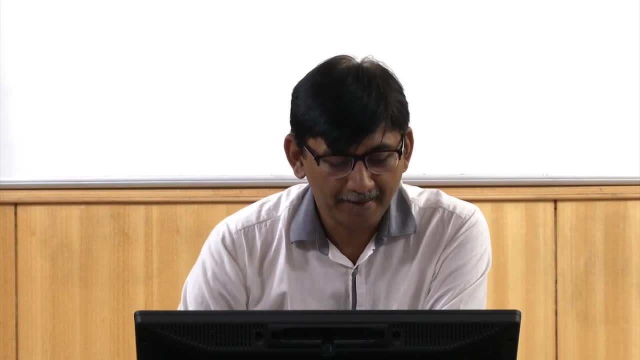 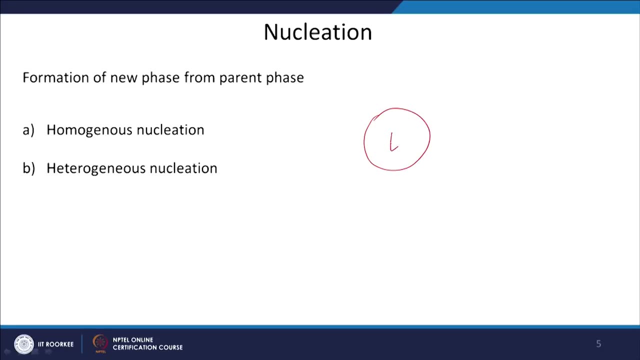 Now, if we come to Nu-cleation, the formation of new phase from parent phase. So suppose I start with a liquid. now the question is where the when I am bringing down the temperature. so I am bringing down the temperature here. so in this liquid, in this system, here, this. 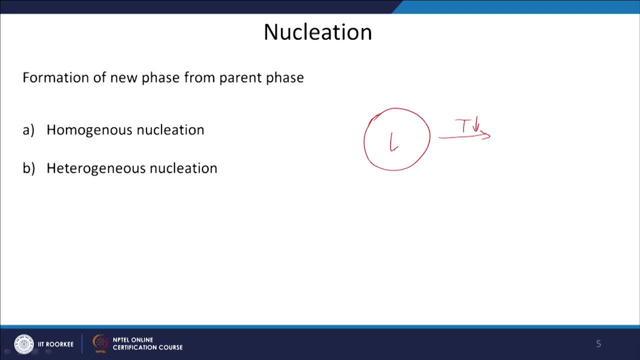 is my system boundary and there is a liquid inside. so where this nucleation is going to take place, is it going to be homogeneous nucleation? that means that the whole liquid everywhere. as soon as I bring down the temperature, at every point there will be some nuclei which 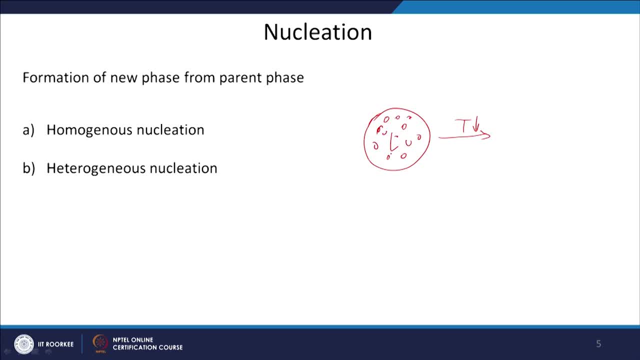 is forming of solid. is it going to be like this or it is going to be heterogeneous nucleation? that means, if this is my system contains the liquid. the nucleation will takes place, for example, at the surface of this system. it can be a vessel or whatever. 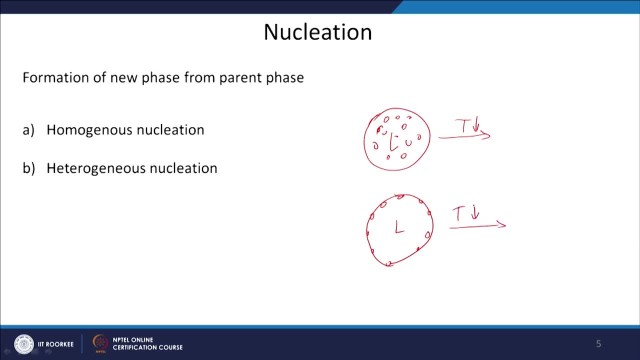 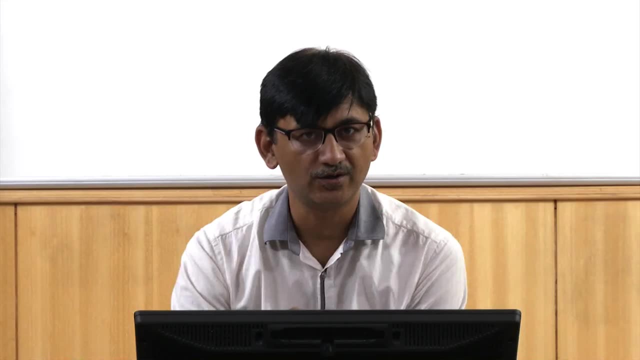 So when I Bring down the temperature here, the nucleation is starting from here. then it will grow inside and later on the whole liquid will transform. so it can be either homogeneous- nucleation means throughout the system the nucleation is taking place- or it can be heterogeneous. 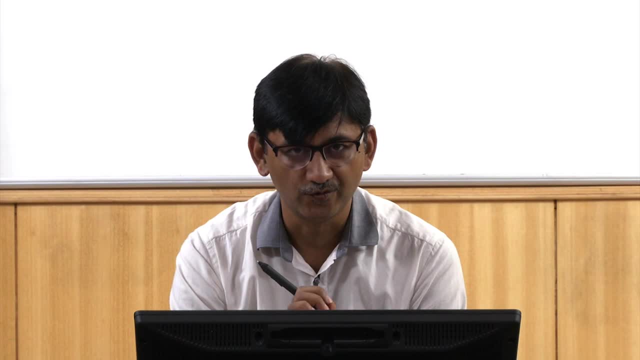 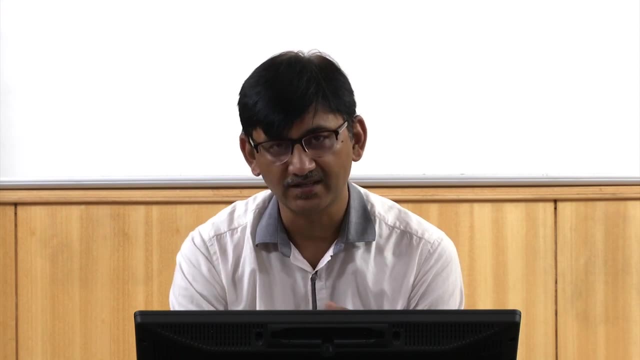 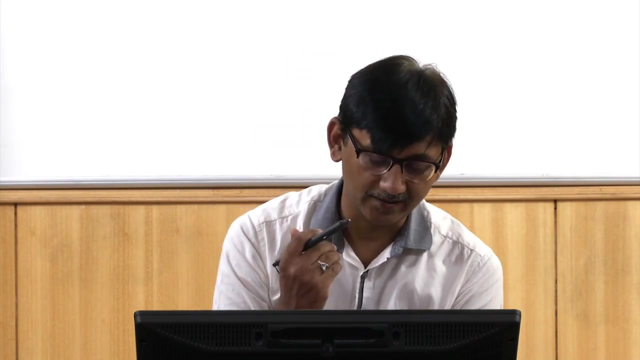 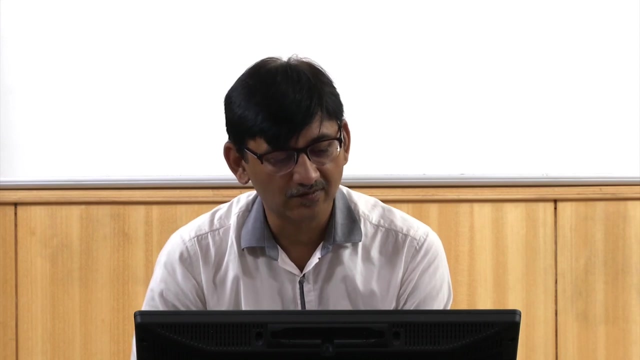 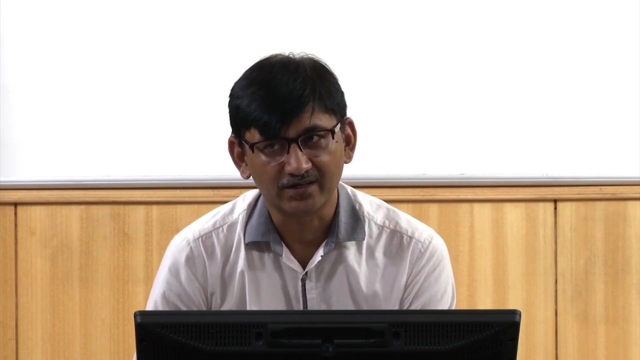 nucleation. that means only at few location the nucleation will takes place. and actually, what decides this whole process? and you will see that most in general, the heterogeneous nucleation is the one which is going to be dominating. to achieve a homogeneous nucleation, actually you have to have very specific conditions. only then you will have homogeneous nucleation. 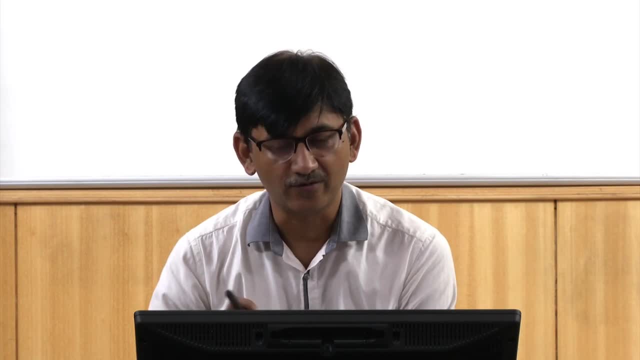 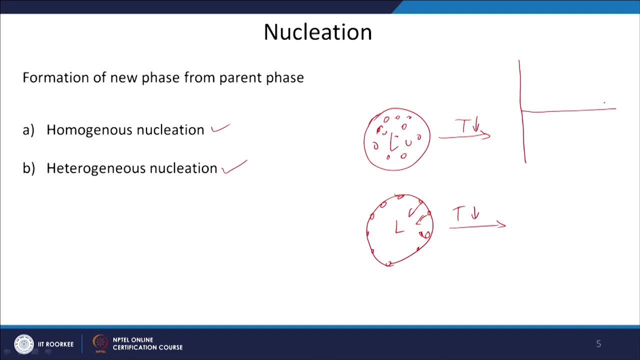 in fact it is a very difficult process to do to have homogeneous nucleation. and the reason is: Suppose, let us say, I draw a free energy curve here, color of the pen here, for example. so suppose you have two axis here. one axis I am saying is axis y, axis is delta g axis. 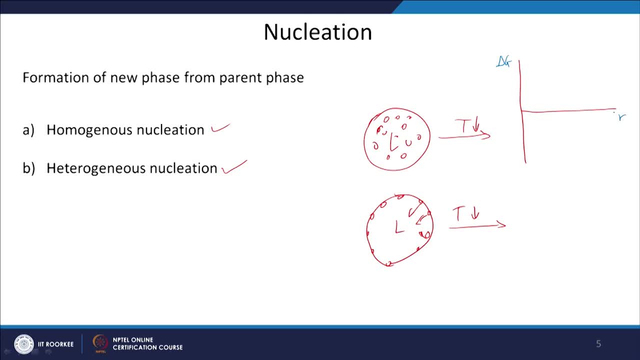 and the x axis is the radius of the nuclei. so delta g is suppose my liquid is not the stable phase. So if I want to go into solid phase, so there is a free energy of the liquid phase and then there is a free energy of the solid phase, delta g will be equal to, let us say it will. 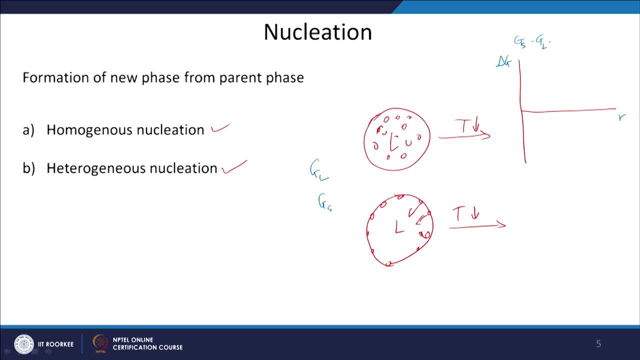 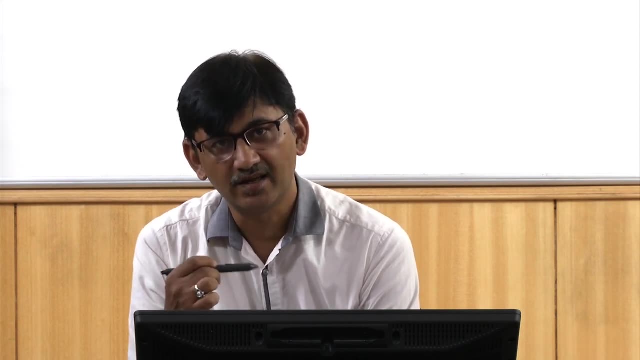 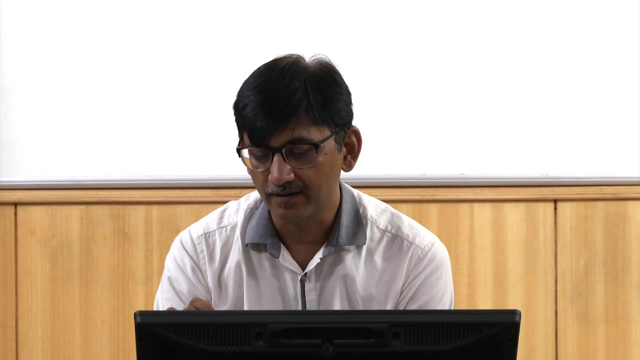 be g s minus g l. so what is the change? in free energy. and if you remember earlier also that we said that the transformation will takes place only when the free energy changes. so the change is negative. So this is at this point, it is 0. and when the transformation will takes place? when the 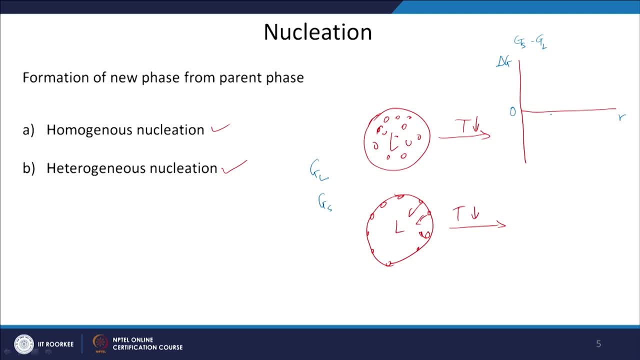 free energy is negative, But the problem is that when you want to have a new phase coming, what will happen? you will have a new interface is there between solid and liquid. so some change is there because of the stable phase is solid now, So there is a decrease in free energy, but there will be also an increase in free energy. 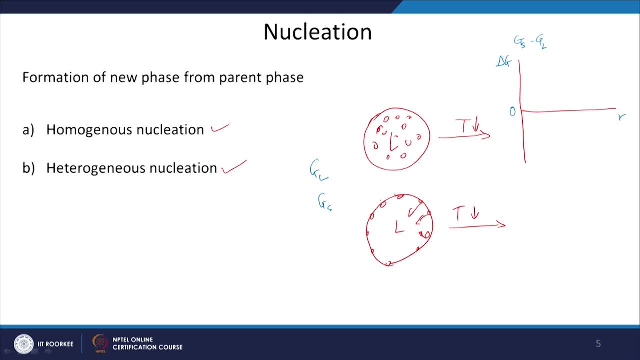 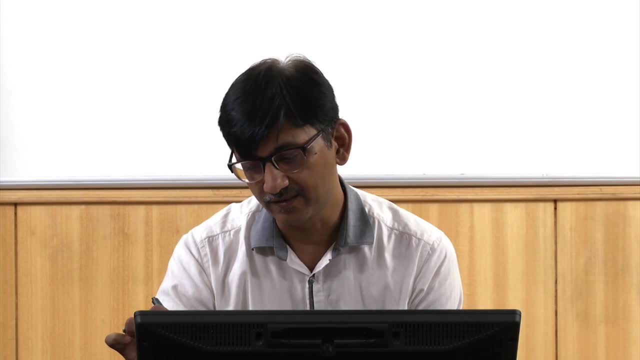 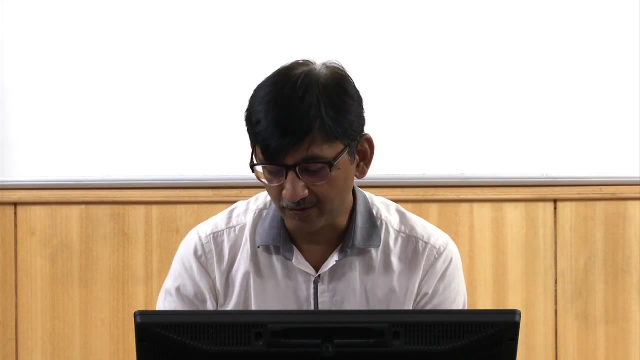 because of the formation of the interface. so all this will? what it does is that it actually increases the free energy initially, and then the free energy decreases as the solid is growing. So as a function of radius, if I want to see, I can have a small nuclei which is forming. 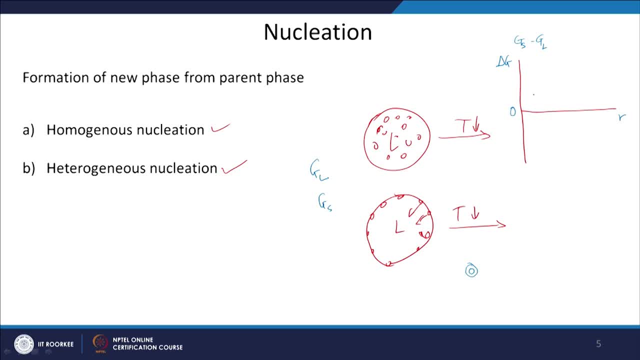 and then it grows and become bigger. So I can draw a free energy diagram like this. my drawing is not very good here, but it will have some curve like this. so you can see that initially, when the transformation is taking place, the free energy is becoming positive and then, after sometime, it is becoming 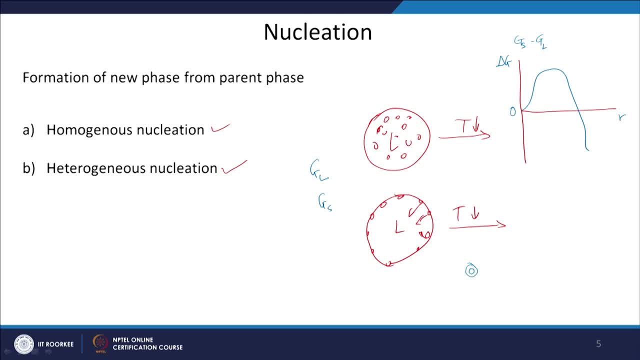 negative. So this increase in the free energy and reaching the maximum will, I will call it as this is known as delta G star, and at the radius at which you have delta G star is called R star. So I will have a stable nuclei only when I have crossed this heel, and this is what 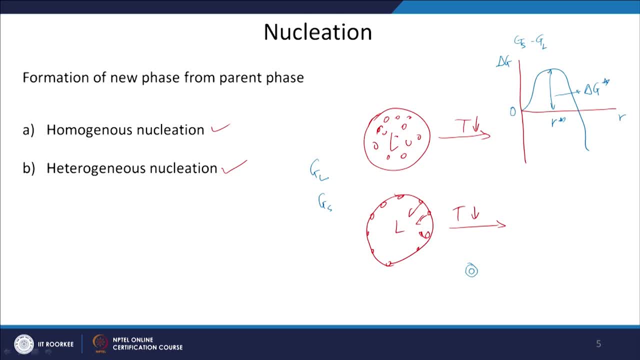 I call as activation barrier. earlier also we use this term. So this is the activation barrier for formation of new phase from the old phase. So this much activation barrier you have to cross to go into the next phase or to have the transformation, and at this point the radius of the your nuclei will be equal to R star. 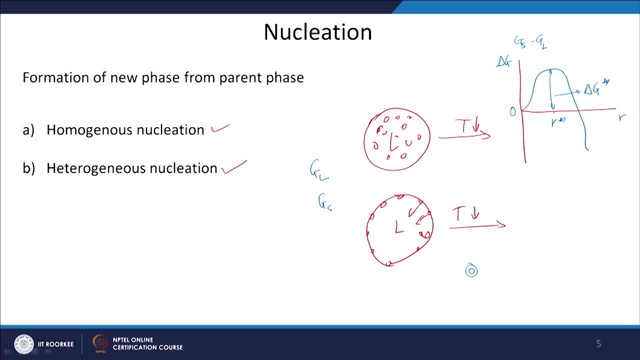 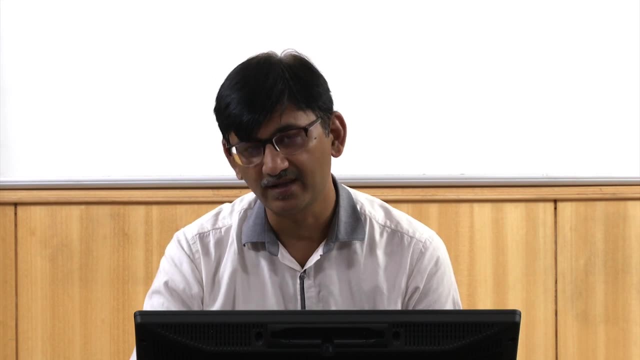 So if I my radius of the nuclei is below R star, then I will call it as embryo. that means it is not a stable Nuclei. it can again go back into liquid phase. If it crosses this critical radius, R star, then it will become a stable nuclei and then 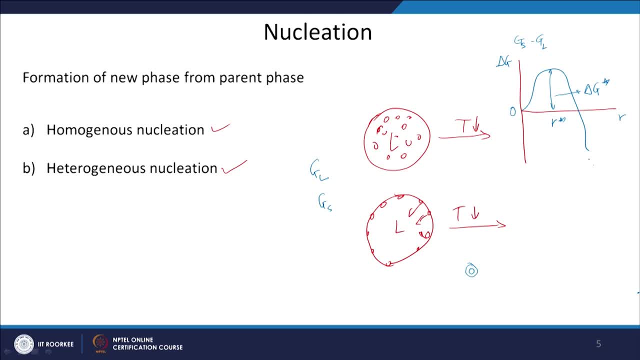 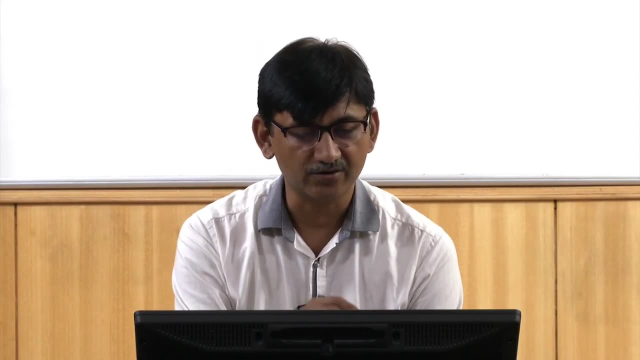 the free energy will start coming down and then it will become negative later on. So this is how the change in the free energy is there. when we transform from one solid to another solid, one phase to another phase, Now how homogeneous and heterogeneous nucleation will come into place. 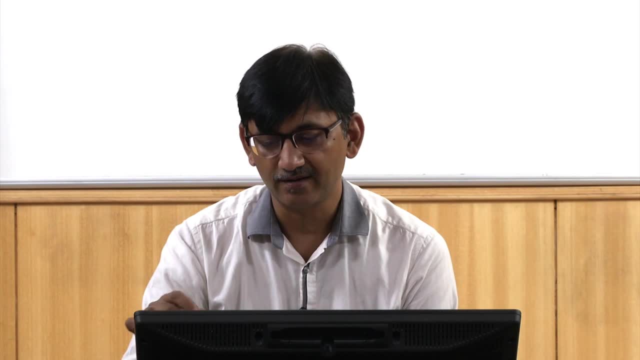 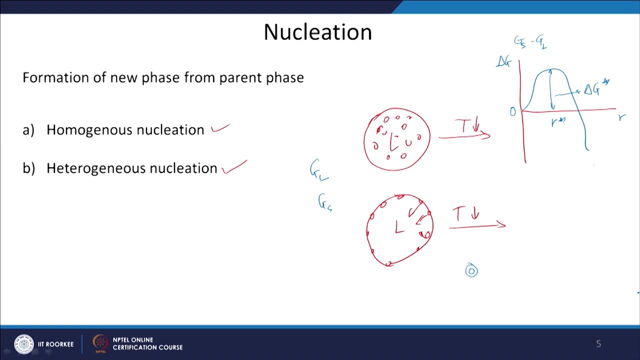 So let us go into picture in this, Suppose this is a curve for homogeneous nucleation, then for the heterogeneous nucleation. for the heterogeneous nucleation, the curve will look something like this: That means the R stars remain the same, but my activation barrier has come down. 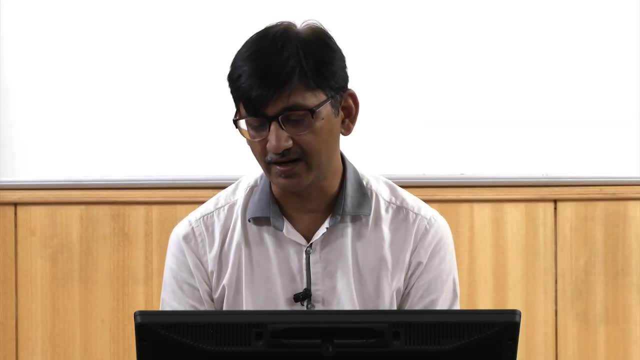 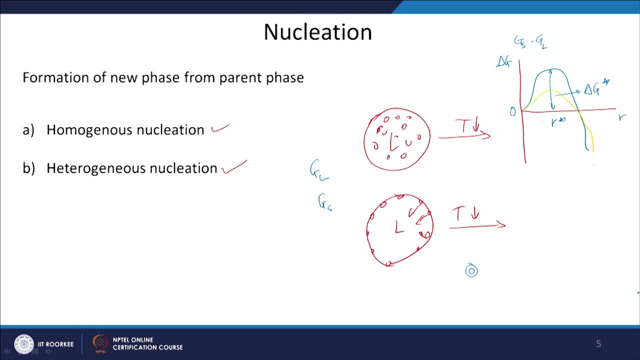 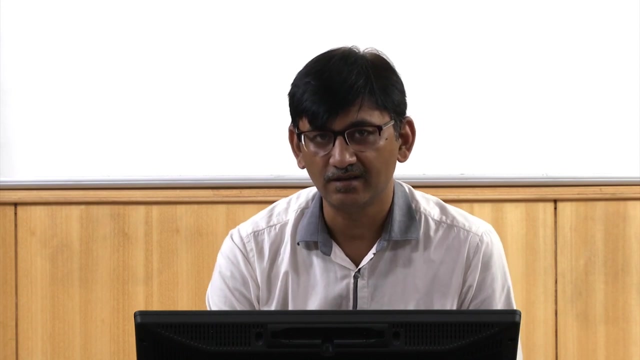 So when I provide heterogeneous nucleation side, what I am trying to do is I am trying to bring the Activation barrier down. Activation barrier down. So I now require a small driving force for changing from one phase to another phase, and that is why heterogeneous nucleation is the dominant nucleation mechanism. when you have 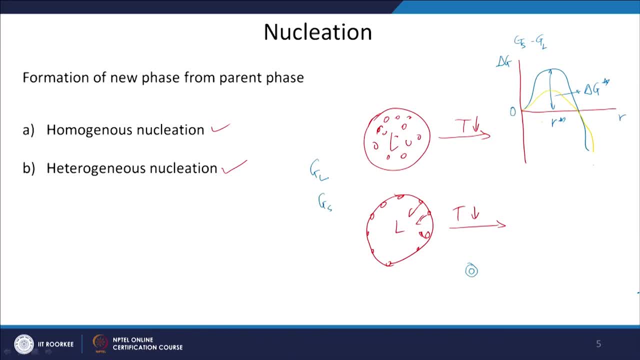 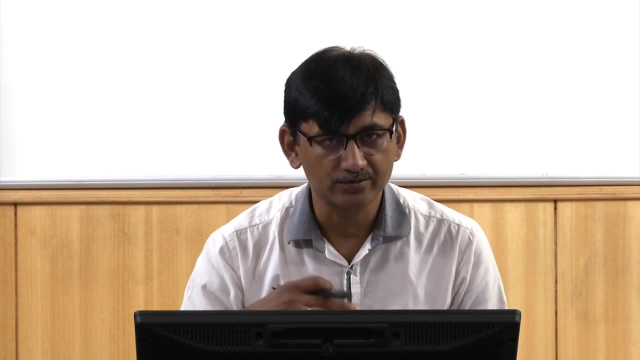 phase transformation. Of course these curves you look into in the books because I have. I am not able to draw it very nicely here. So if you want to look at heterogeneous nucleation sites, Ok, Of course I am not talking about solidification now. I am talking about in transformation, in. 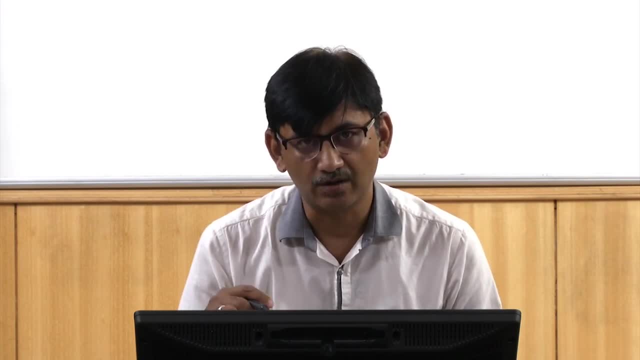 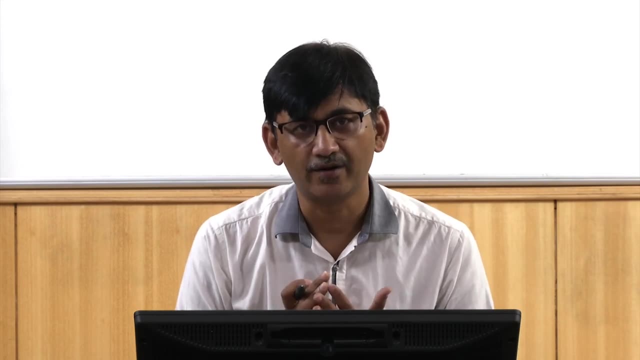 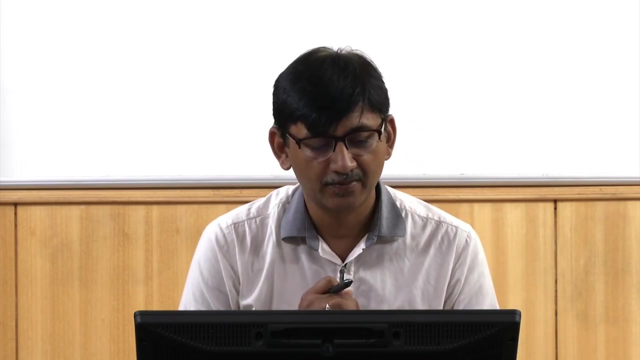 solid phase. when you talk about the transformation from liquid to solid, the vessel wall is a very good nucleation site. If there are some foreign impurity particles are there, then they can act as a nucleation site when you have transformation. So this is solid to solid transformation. 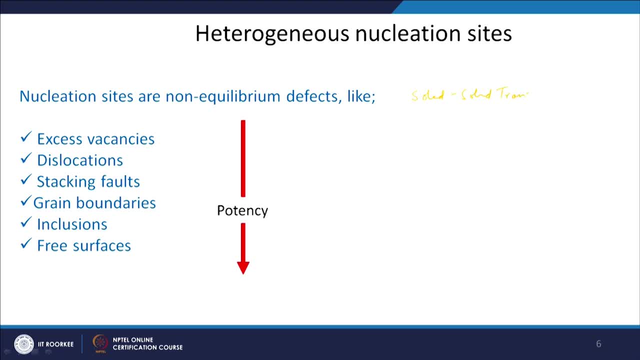 So in this case we are talking about solid to solid transformation. So nucleation sites are the non-equilibrium defects. So you have a either excess vacancies, vacancies are equilibrium defects, but when you have excess vacancies more than the equilibrium vacancy concentration. so of course that 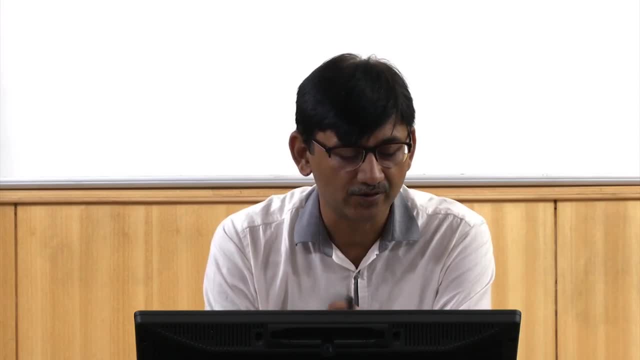 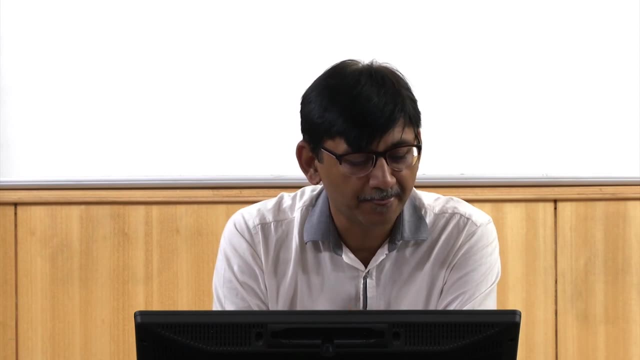 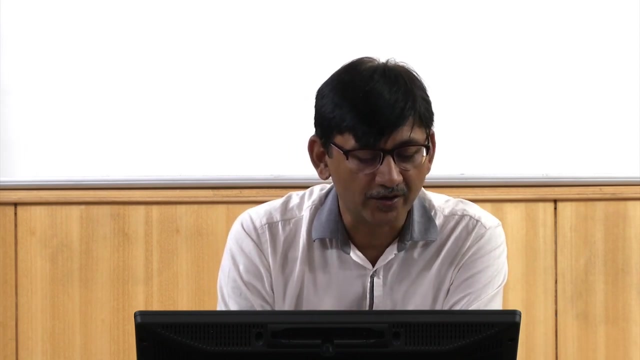 is not a equilibrium condition, So then we will call it as non-equilibrium defects. Otherwise, equilibrium vacancy defects are the equilibrium defect, that is, thermodynamically it is a vacancies have to be there, So excess, if you have excess vacancies, they can. they that can act as a heterogeneous nucleation. 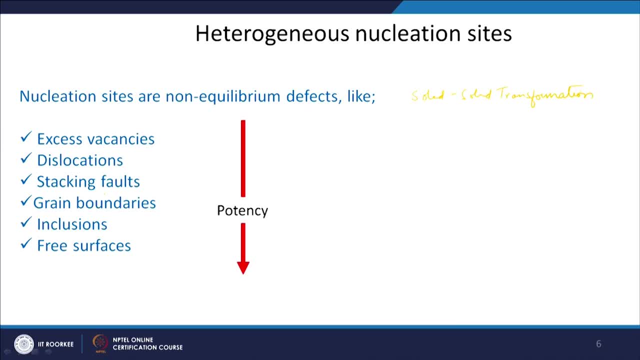 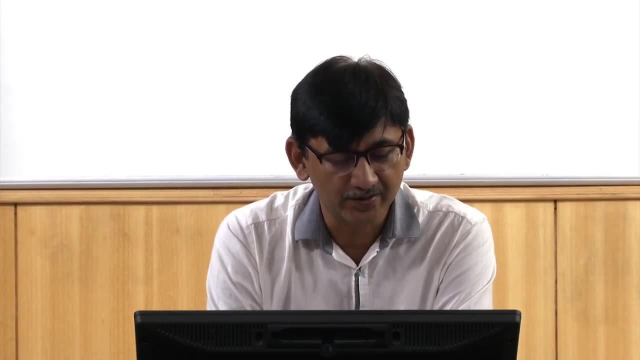 site dislocation can act as heterogeneous nucleation site staking. faults: are there grain boundaries? are there Inclusions? are there already? inclusions are present on which you can have another phase forming, or you can have free surfaces on which the nucleation can takes place. 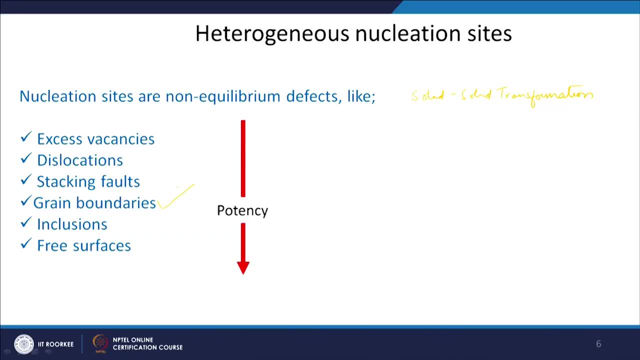 Out of this, the grain boundary is one of the most important nucleation site because first thing is that it has very good potency. you can see the potency of the nucleation site is increasing. So free surface is the most potent site and excess vacancies are the least potent site. 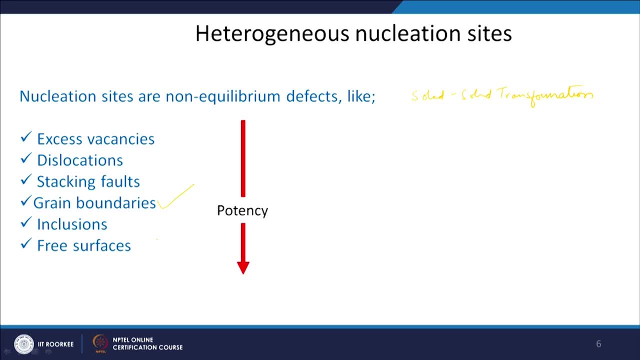 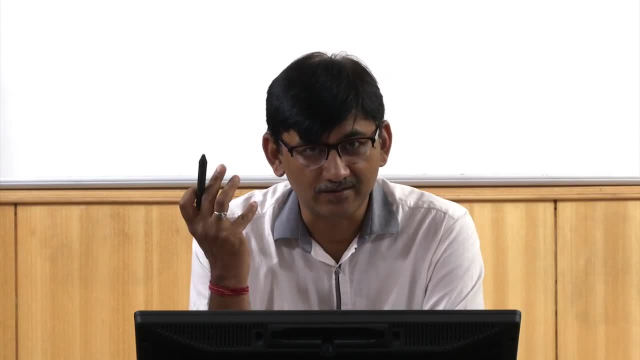 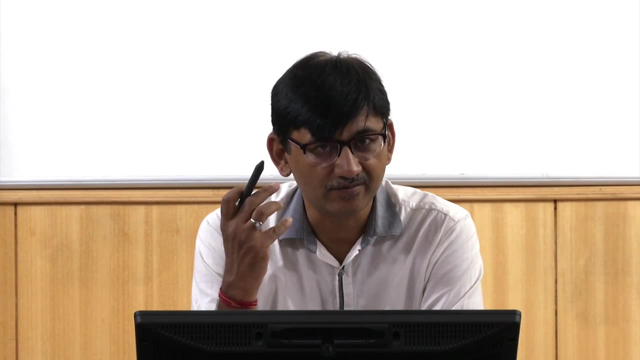 So grain boundaries are highly potent. and the second thing is that in the material there are large number of grain boundaries, So the, if you want to see the concentration of the sites, the grain boundary sites will be of in very high concentration. Inclusion in free surface: free surface can be only on the outside. 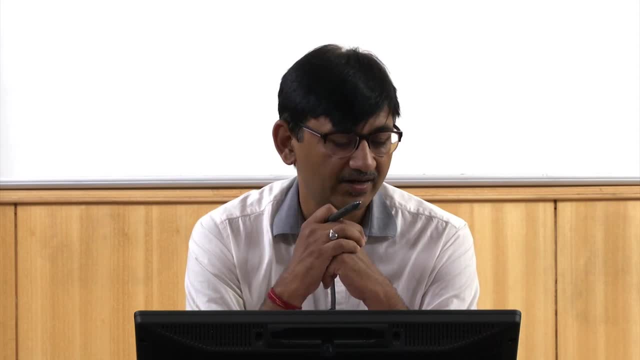 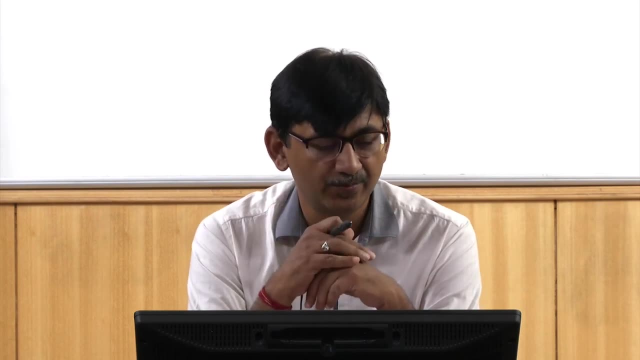 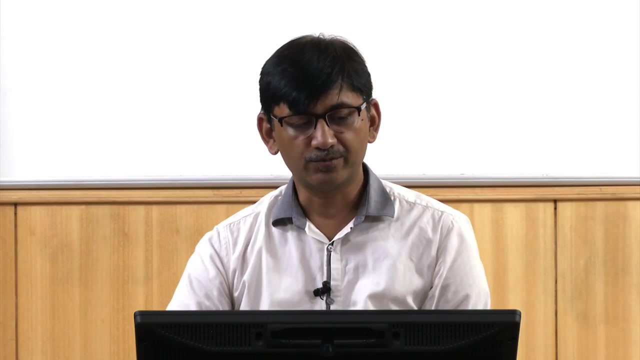 So for a given volume, the amount of free surface will be very less. Inclusion also if your material has impurities and then inclusions will be there. So the grain boundary is actually one of the most important heterogeneous nucleation side. Now coming to coming to growth, the growth is given by a equation called Johnson-Mahal-Avarami-Kolmogorov. 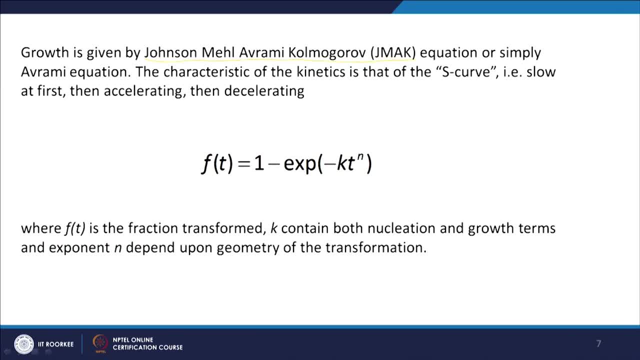 equation, JMAK equation, or simply we called this, is a Avarami equation, and the characteristics of this is that is that Nope is there. it gives you a typical S curve, which what it shows is that the growth kinetics are slow, initially at first, and then it accelerates and then, at the end, it decelerates. 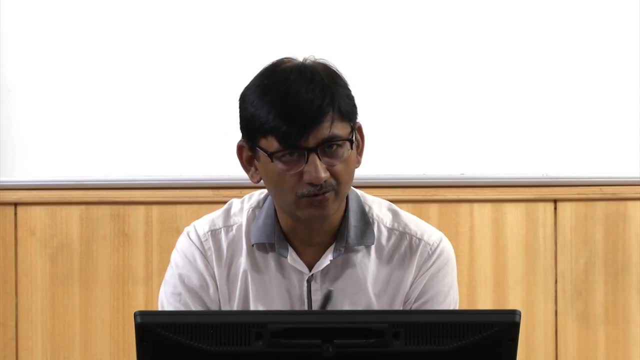 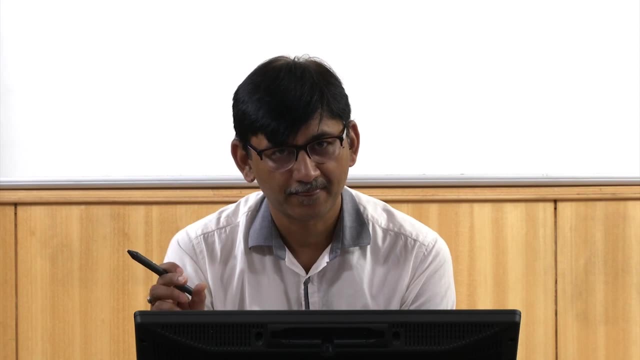 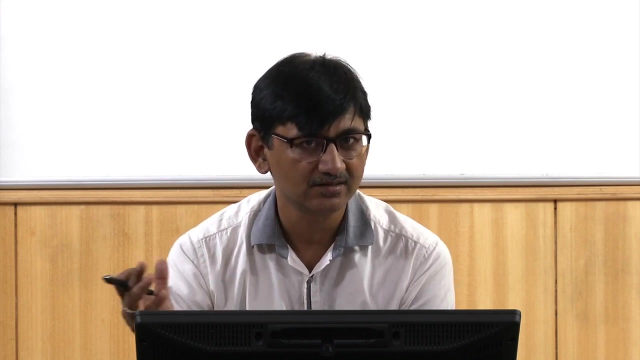 So this is the typical growth kinetics you will find out in large number of systems. For example, if you want to see a bacterial growth, then also you will have similar S curve. ok, So S curve you will see in large number of different systems, so it is a very common system. 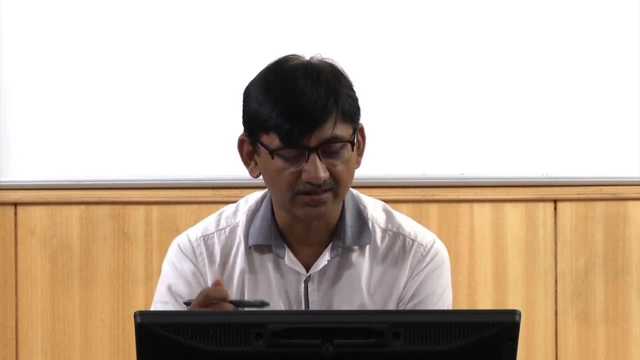 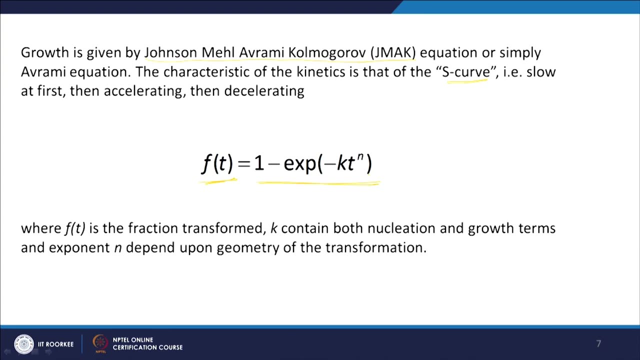 or common characteristic and it is given by an Abrahamian equation and the fraction as a function of time will be given by an exponential expression like this, where F, t is the fraction transform, k contain both nucleation and growth terms and exponent n depend upon geometry of the transformation. ok, 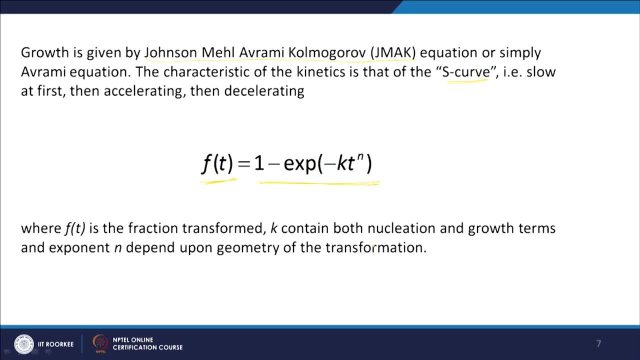 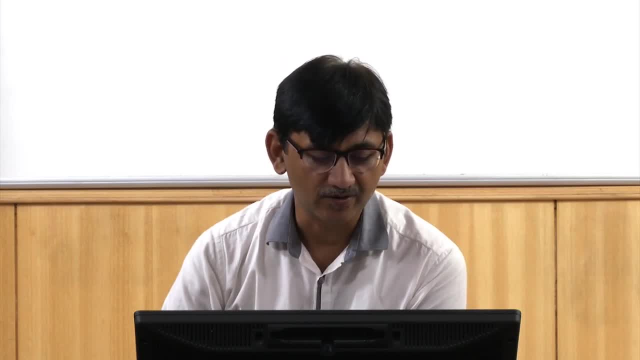 So you do not have to worry about that. So all these things will come into the overall growth kinetics. So this is what your typical S curve will look like. So this is on the x axis, you have fraction transform ok. 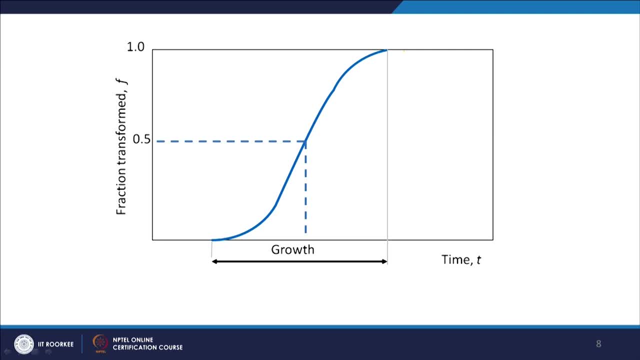 So one means it is fully transformed, 100 percent transform. ok, There is some gap up to which time you would not have any transformation. so this is you can understand as a nucleation. So this is the nucleation gap. then this is the first. it is slow, as we told you, then it 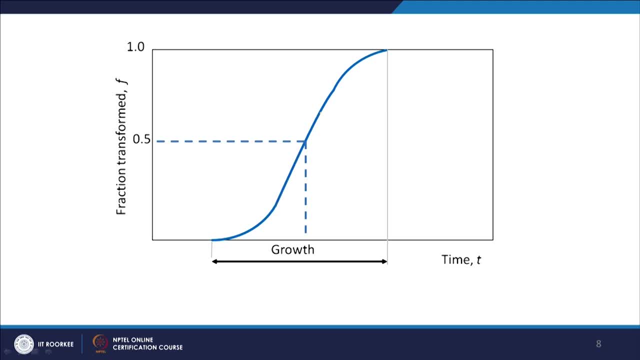 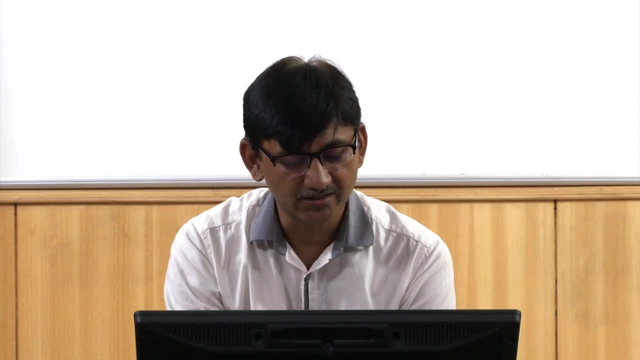 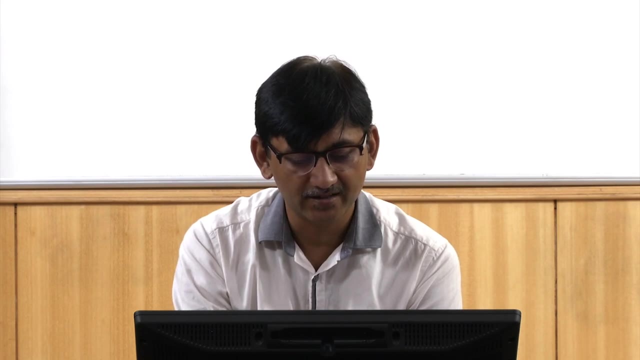 accelerates, ok. then it becomes, goes into a steady state condition and then it decelerates and become very slow at the end also. So initially also it is slow and at the last stage also it is slow and it has maximum growth kinetics in the in the, this central part, ok. 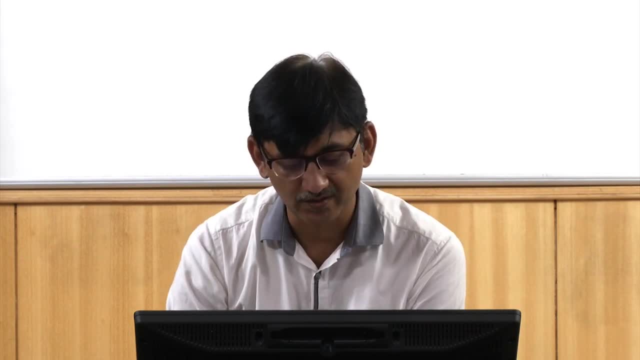 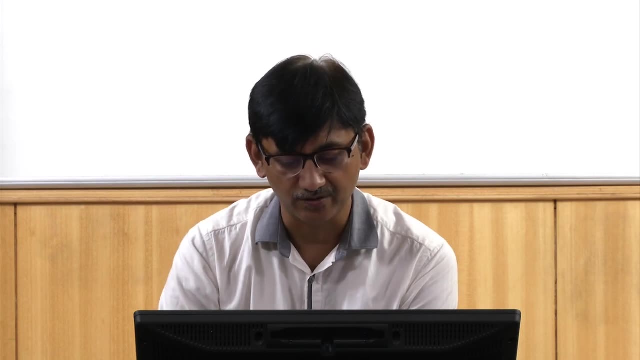 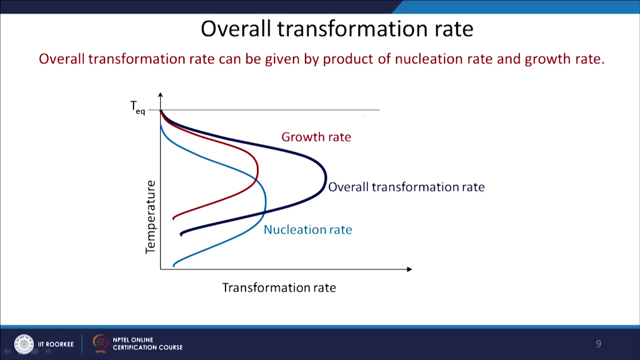 So it is. So this is typical S curve. you will usually see in lot of transformation one of, and you will see it in the our phase transformation also. So, as a function of time, what is the fraction transform is what is shown here from that. 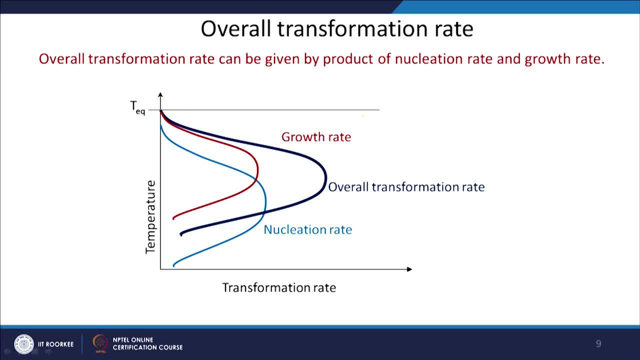 from the idea of nucleation and from idea of growth, I can- we can say that you will have some rate of nucleation, So this 18.. tied equilibrium temperature: ok, below which the phase transformation will start. ok, So nucleation will start after you do some amount of under cooling. ok, So I use this. 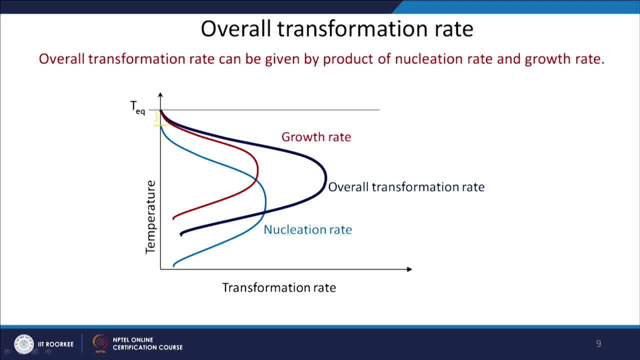 word during solidification also. So some amount of under cooling will be required. under cooling. why we have to have under cooling: ok, to provide driving force for nucleation. Why we need driving force to overcome activation barrier: ok, So there is always going to be some under cooling is required to start the transformation. 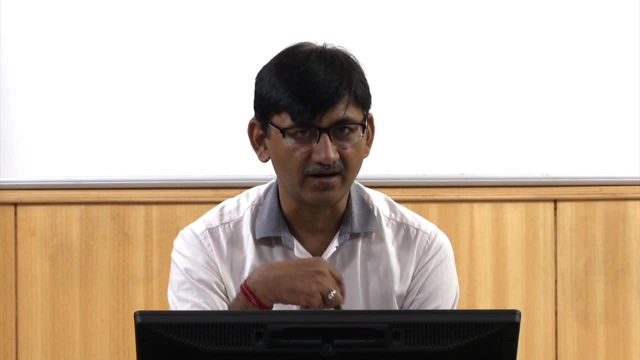 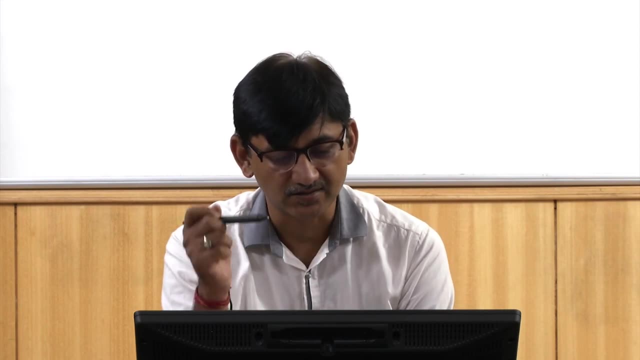 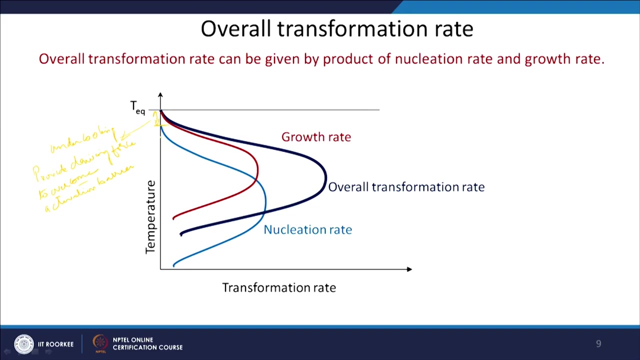 ok, That under cooling will give you the driving force for transformation and that driving force is required to overcome the activation barrier, as we just discussed. ok, So this is your nucleation kinetics. So initially it will be, there will be some under cooling.